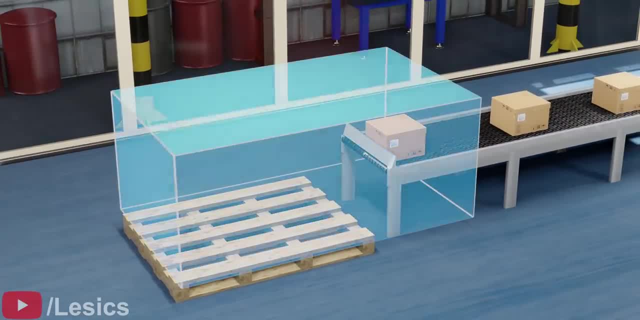 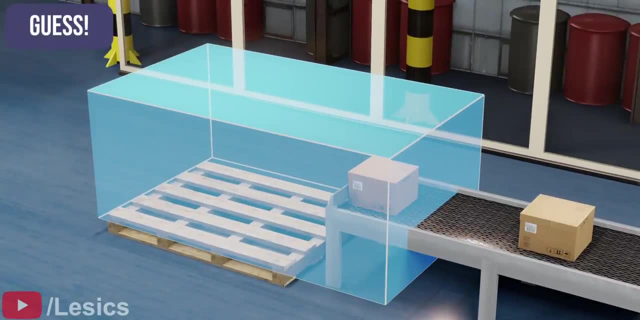 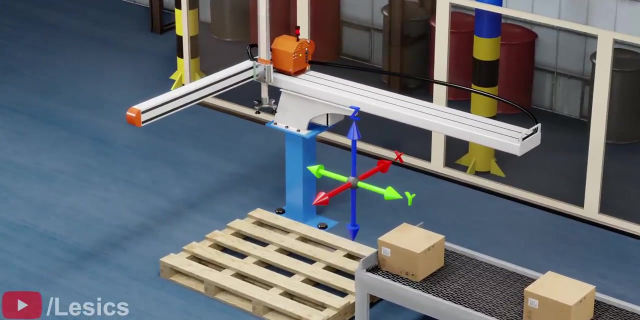 The work envelope required for the robot is obviously rectangular in shape. Can you guess what type of robot configuration is the best fit to complete this task? Yes, you'd need a robot with linear motions in all three directions inside this volume. This robot has three linear joints to accomplish movement in the X, Y and Z directions. 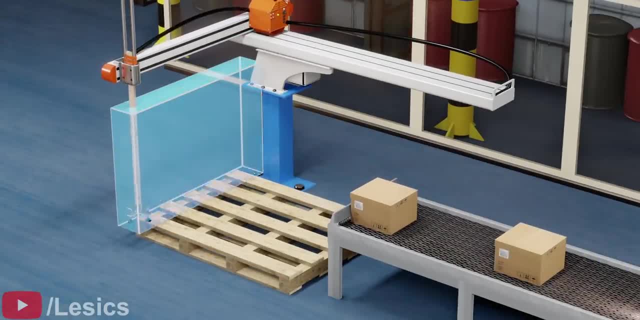 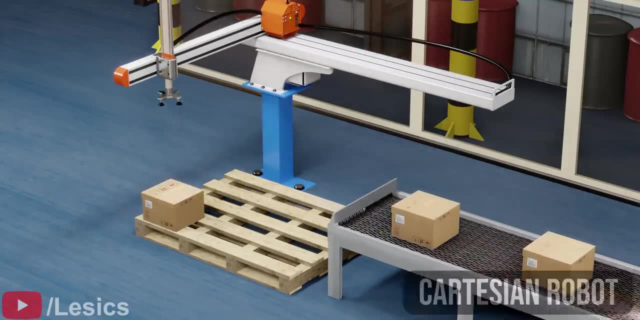 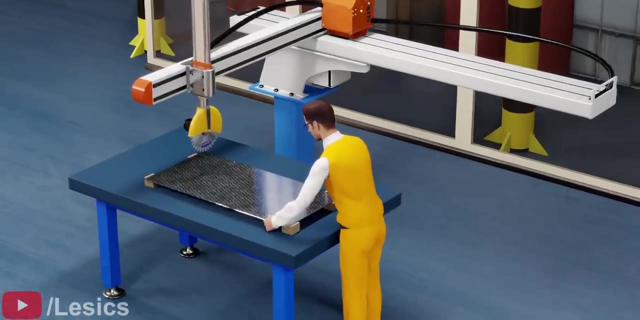 This robot's end effector can pick up the object anywhere inside this rectangular work envelope, move in all three axes and place it as needed. These kinds of robots are called Cartesian robots. Now let's consider the same robot, but this time it's using a different end effector, a metal cutter. 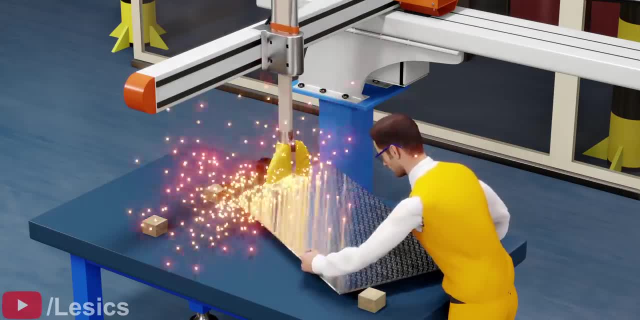 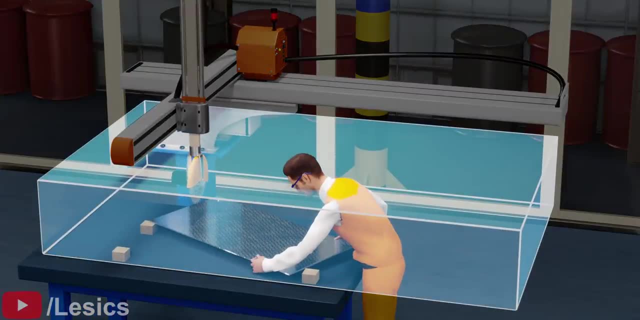 Here, due to the nature of the work, the operator has to be inside the work envelope we defined earlier, which can be highly dangerous For safety purposes. you won't want this new end effector to go near the operator's hand. In short, 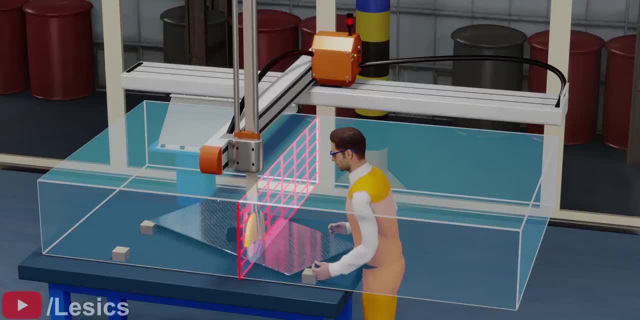 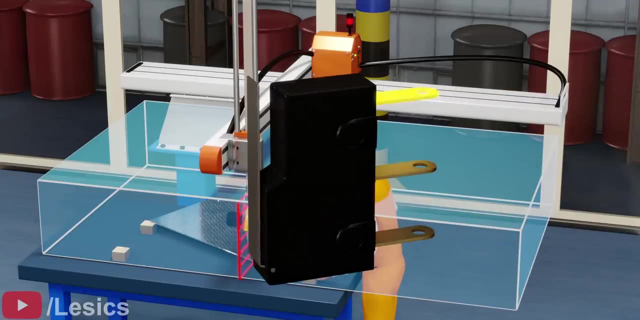 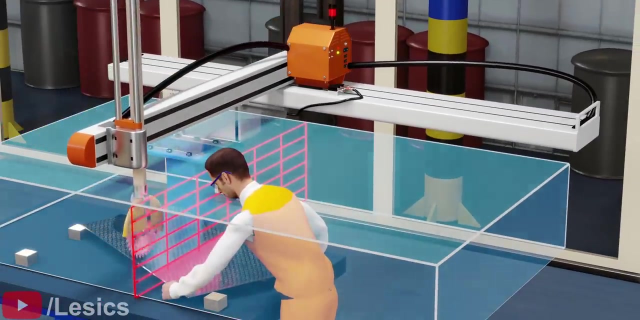 block the robot's movement in the Y direction after this red plane. To achieve this end, engineers often restrict the movement of the robot by using electromechanical limit switches, which creates a border beyond which the bot cannot go in any given conditions. In short, 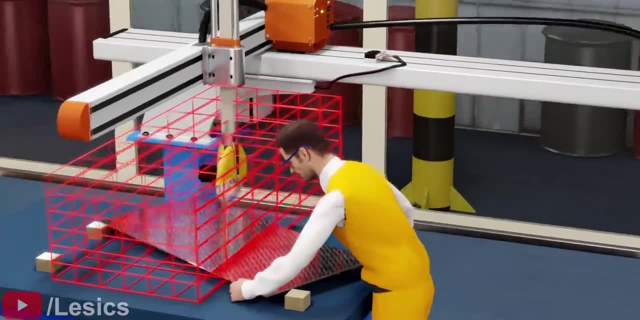 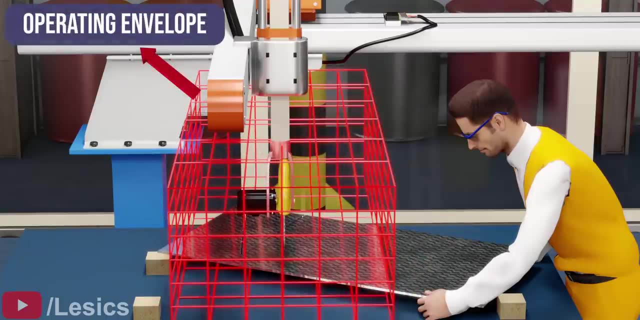 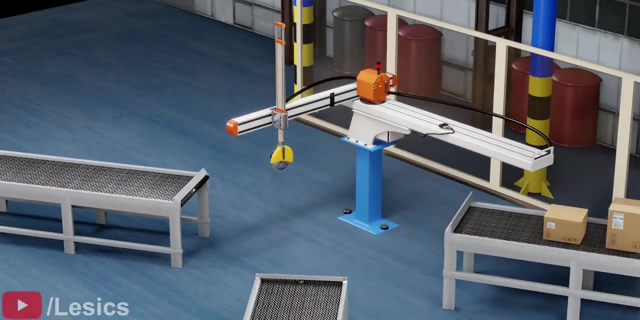 even though the work envelope is huge, this robot will be able to work only within this red volume. This new red volume is called an operating envelope. Let's move to our next robot and study a different work envelope. Let's assume that the robot has to move these boxes from one conveyor belt to another. 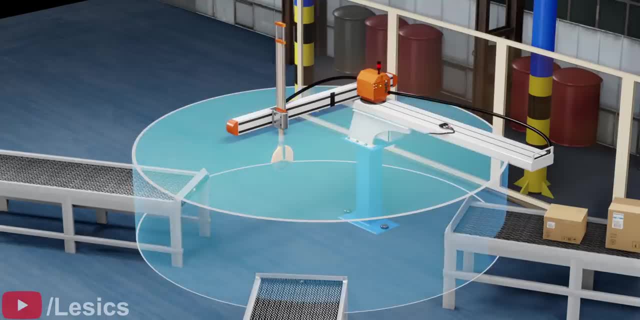 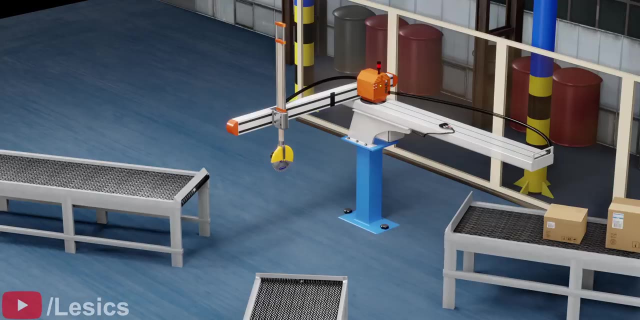 The work envelope needed for this task is obviously cylindrical in nature. Can you suggest some design modifications to the previous robot to achieve the new work envelope? To attain the cylindrical volume, we need two linear movements and one rotary movement. Simply replace one linear joint from the Cartesian robot with a rotary joint. 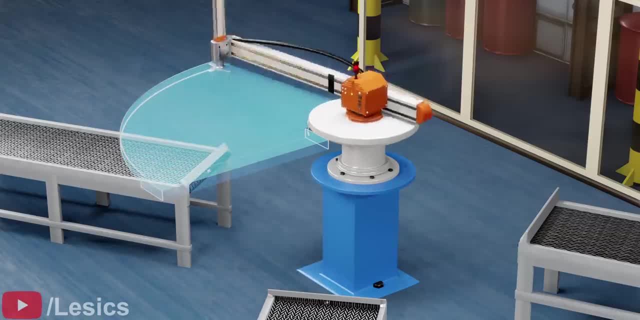 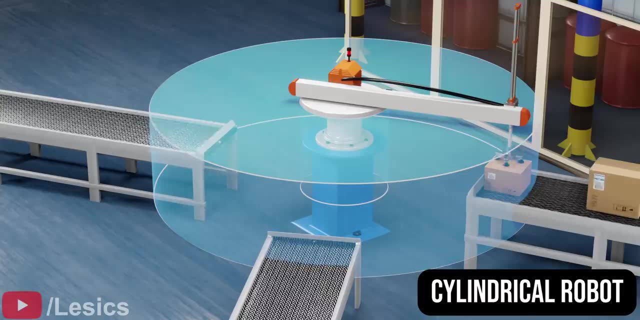 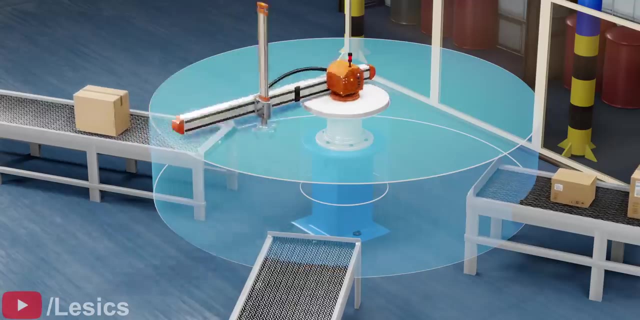 Now the robot can rotate 360 degrees on its central axis. These kinds of cylindrical robots are mainly used to work as mediators between two or three massive machines to transfer an object from one station to another. If you observe carefully, you can see that. 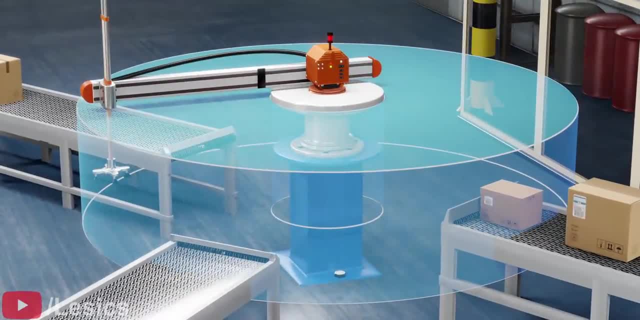 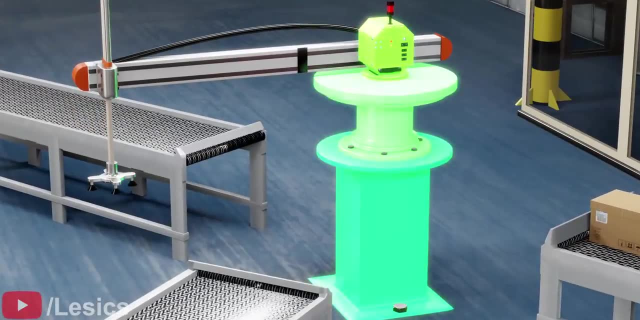 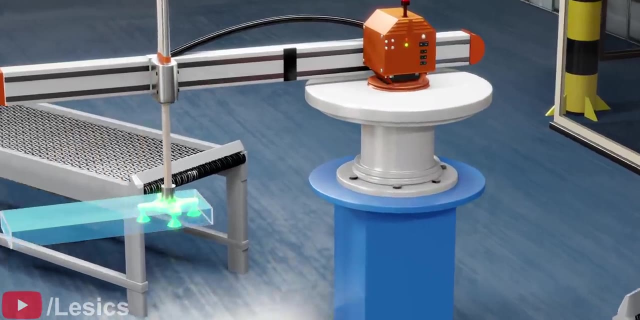 the work envelope here is not a solid cylinder. It has a dead zone at the center. Can you tell why This dead zone is due to the robot body's physical limitation? In this case you can see that the robot's arm can retract only up to its body and not beyond that. 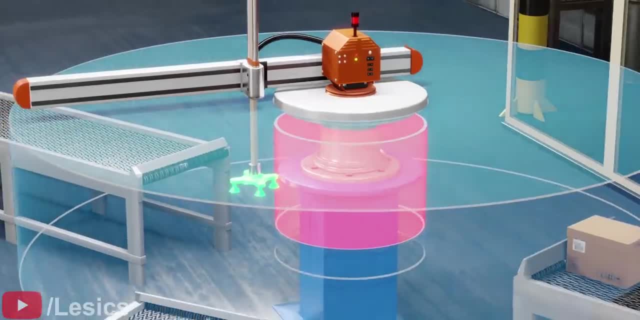 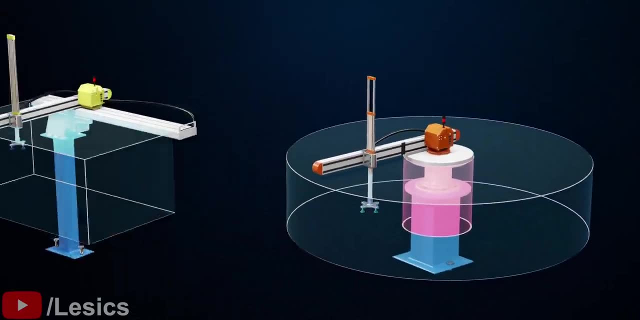 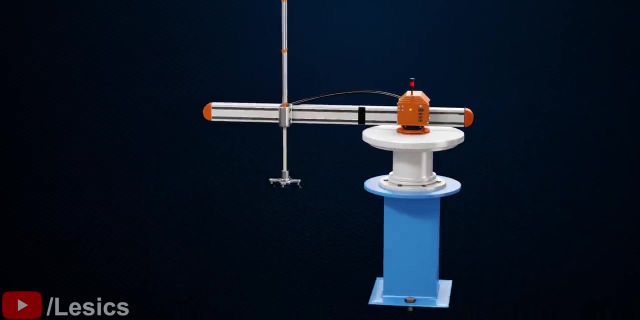 Thus, a dead zone volume will always be inside the cylindrical robot's work envelope. However, such dead zones are not present inside the Cartesian robot's work envelope. With a simple design modification, we can convert this cylindrical robot into a more versatile robot which does tasks like welding this car chassis together. 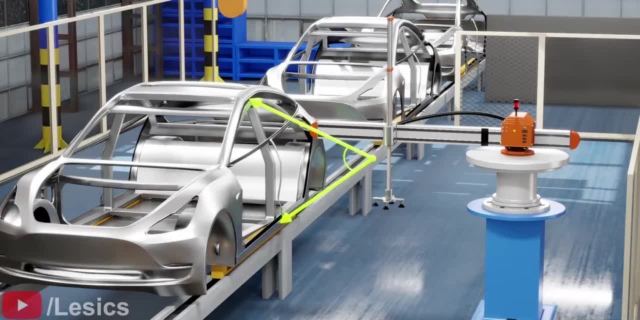 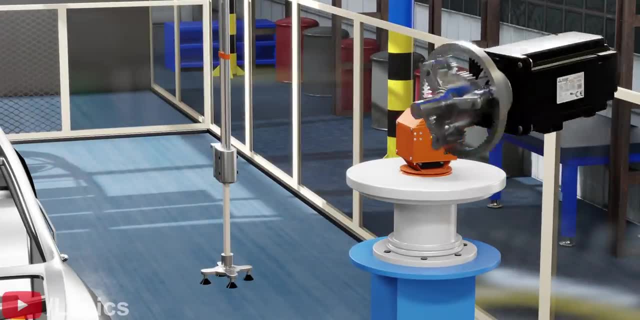 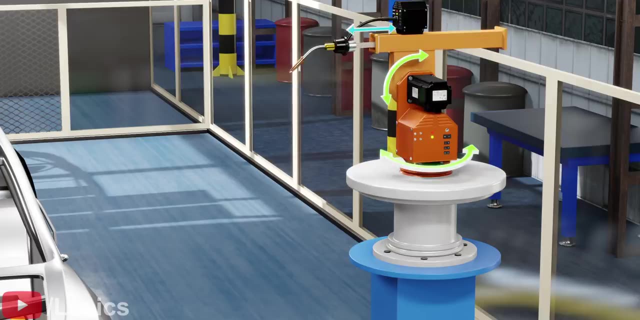 For this task, the robot has to turn at different complicated angles. The cylindrical robot cannot perform this task. All you have to do to achieve it is replace one more linear joint with a rotary joint. Here. this rotary joint can go from approximately positive 30 degrees to the bottom of the ground. 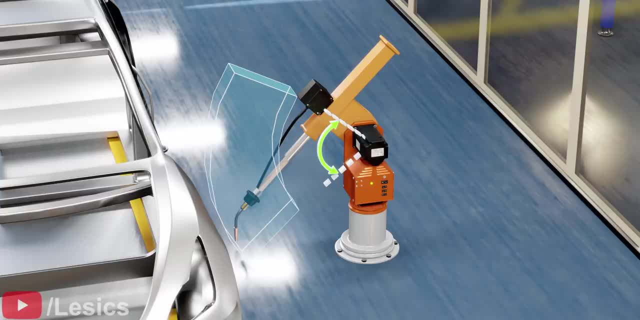 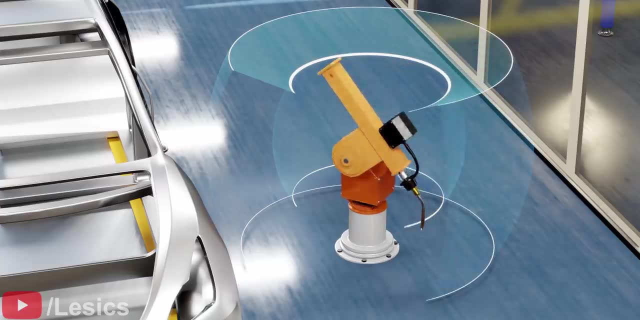 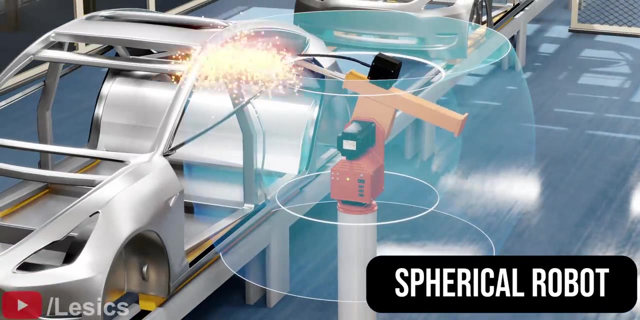 Now, using your visualization skill, can you predict this robot's work envelope? Just revolve this shape 360 degrees in the z-axis. What you get is a partially spherical work envelope. These kinds of spherical robots can easily complete this welding task with an angle. 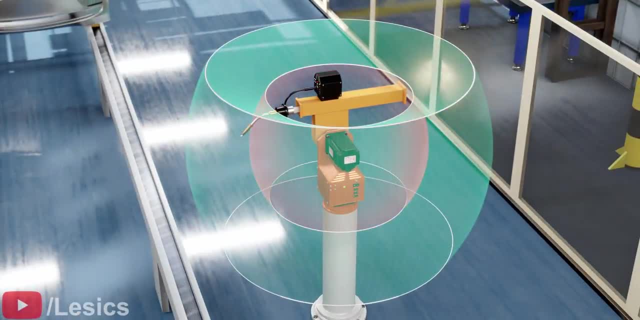 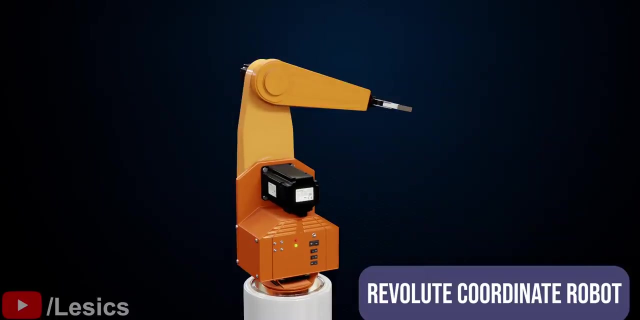 What you see in the central area is the dead zone of a partial spherical configuration. This space can be an efficiency weakness. If we replace the last linear joint from our robot with another rotary joint, this will make it a revolute coordinate robot, which should reduce the dead zone and give the robot more reach. 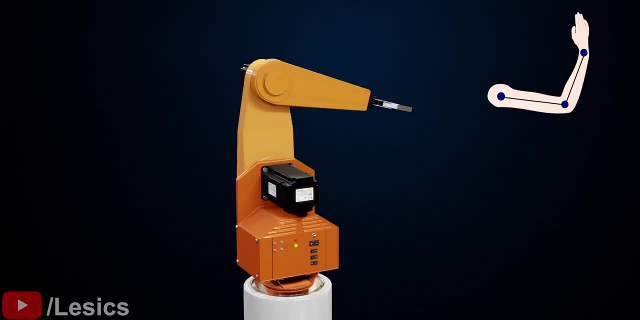 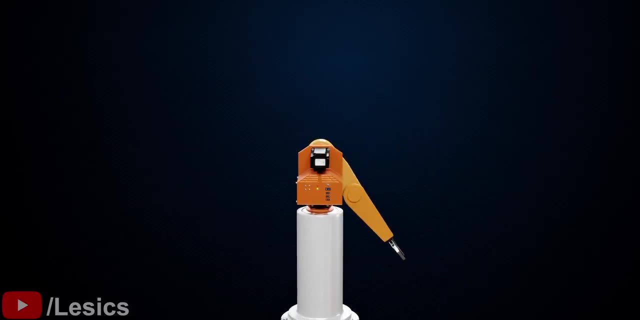 This robot looks similar to a human arm. right Now the new challenge. Let's deduce its work envelope. First, let's freeze the z-axis rotation and figure out the 2D work envelope which arises due to the robot's remaining two rotary arms. 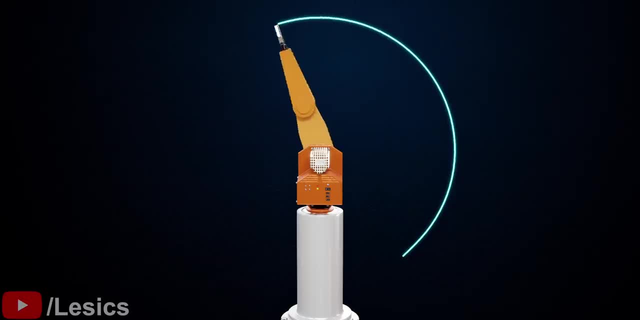 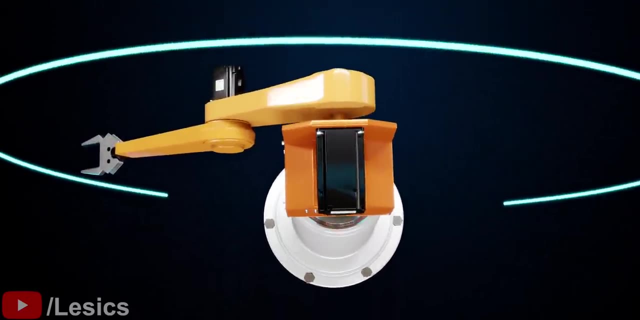 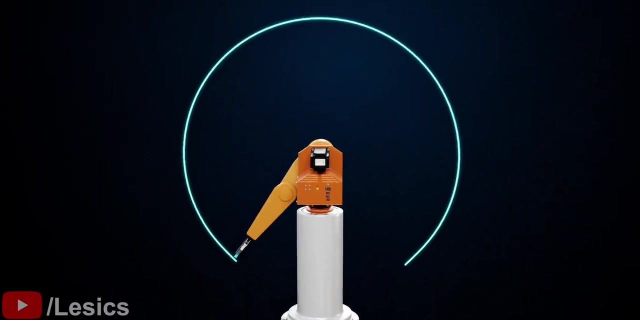 When both the arms are fully stretched, the end effector can draw a circle of 280 degrees. You can observe from the top view why this joint cannot go beyond this 280-degree angular limit. Anyway, this is the biggest circle this robot can draw.